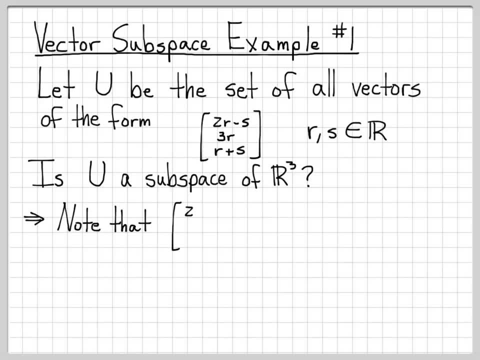 That's the question that we're asking here. So one thing that we can note is that we can actually rewrite this vector in a certain way. We can rewrite this vector as r times the vector 2, because there's a 2 right here. 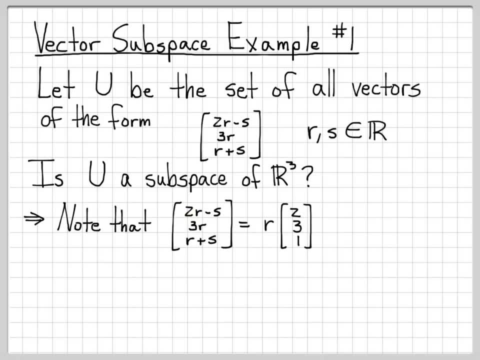 As the second element. we can put a 3 there and 1 is the third element, And then we can add s times the vector negative 1, 0, and s because there's a negative 1 here in terms of how many s's there are. There are zero s's here. 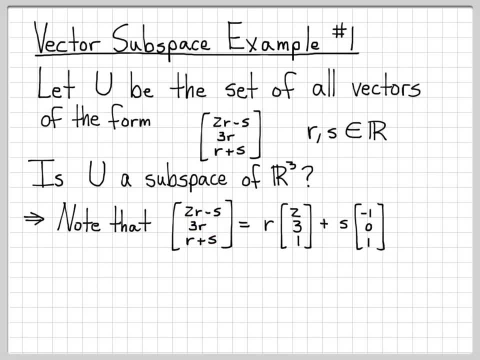 And there is one s right here. So one thing to note is that this vector that we're working with kind of this general form can be factored as this linear combination in terms of r times the vector plus s times the vector. And one thing that's interesting to note is that both of these vectors, 2, 3, 1, and 1, 0, negative 1, both of these vectors are actually elements of r3.. 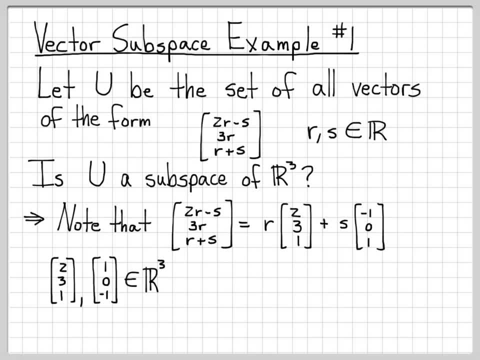 And that fact alone helps us solve this problem in terms of determining: is U a subspace? Is U a subspace of r3?? Another thing to note is, since we've been able to write U in this form, we've been able to write U as r times a vector plus s times a vector for all values of r and s. 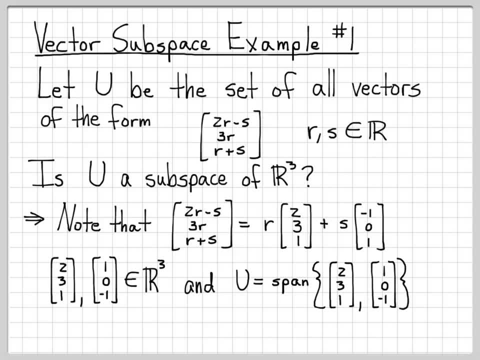 By definition, we've been able to write this: set U as the span of these vectors, because remember what the span means. Span means: take all linear combinations of the vectors. Well, that's exactly what we have here. r and s are arbitrary scalars from the reals. 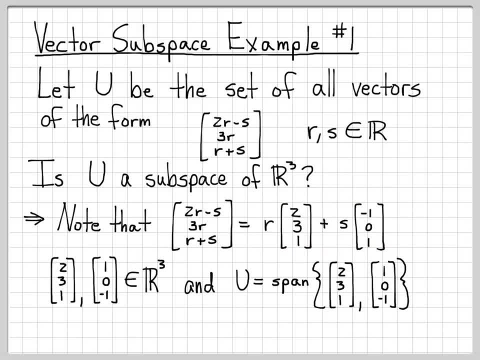 So it's It's very clear that we can write U as the span of these two vectors, 2, 3, 1, and 1, 0, negative 1.. So how does this information help us establish that U is a subspace of r3?? 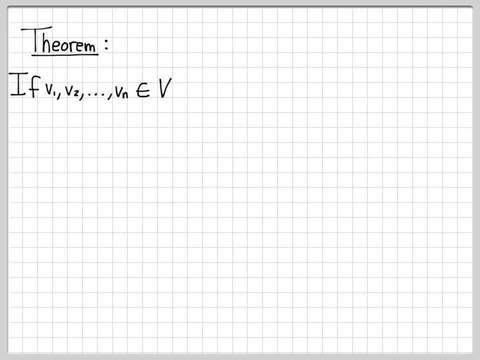 Well, there's a theorem that helps us do this. There's a theorem that says: if you have vectors v1,, v2, all the way up to vn, so some set of vectors, and they are in the vector space v, so you're working in some vector space v.